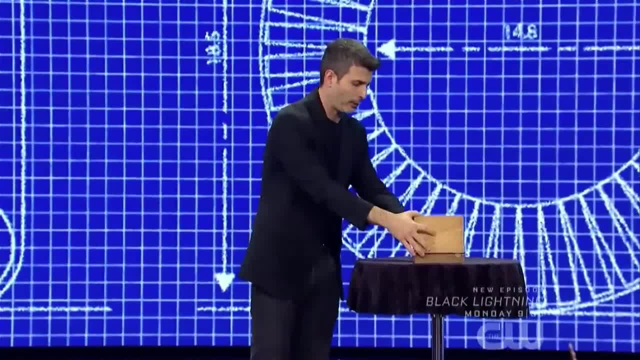 Spades, Spades, and you switch to king of clubs. Very, very, very interesting Because I have, as I told you, a deck of cards Before the show: backstage I have a deck of cards. Before the show: backstage, I have a deck of cards. 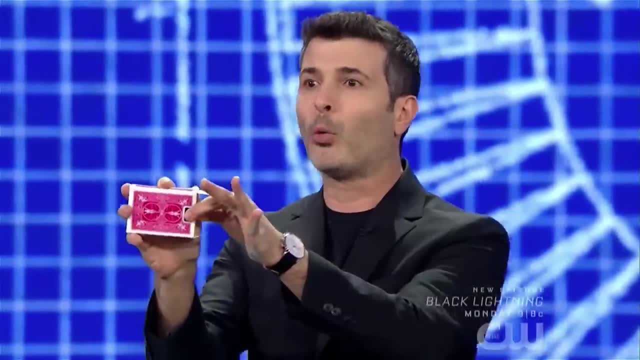 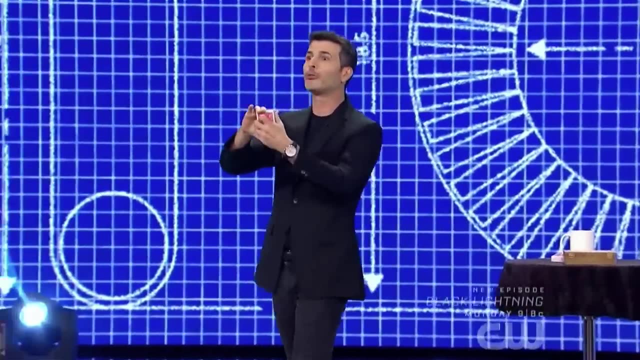 Before the show, backstage, I went through the deck and I removed one card from the middle and reversed it, And it could have been any one of these, obviously any one that you named, But you named the king of clubs. 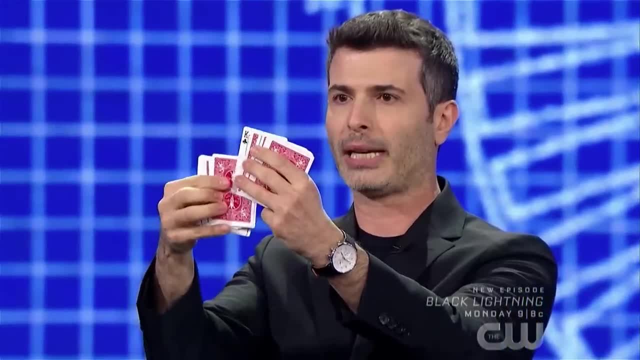 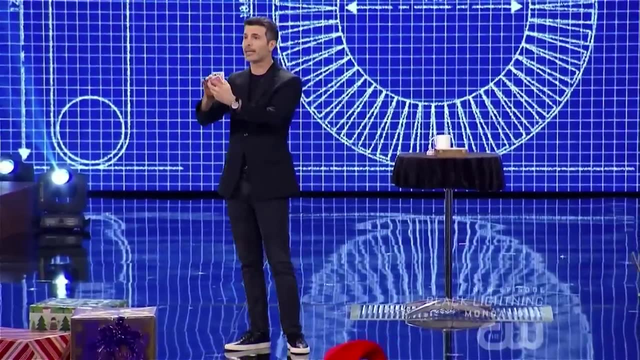 And I'll show you every single card, every one of these, except for one card in the middle is the king of clubs. No, no, no, no. I was really sure you were going to say king of clubs, that I took this card from a different deck. 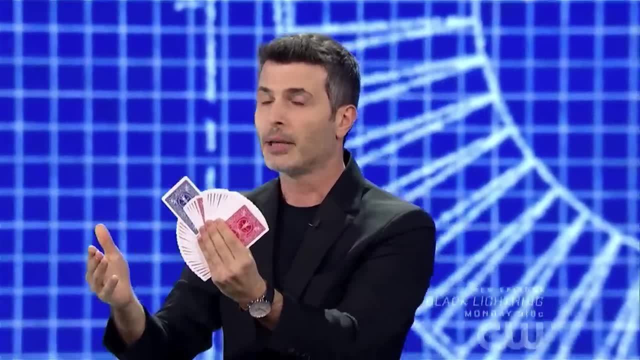 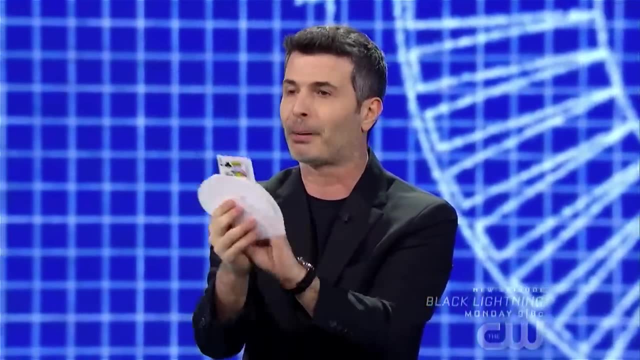 That's how sure I was. It's the only blue card in the deck. No, no, no, I was really sure I don't have any other card but the king of clubs. It's the only card I have here. These are all blanks. 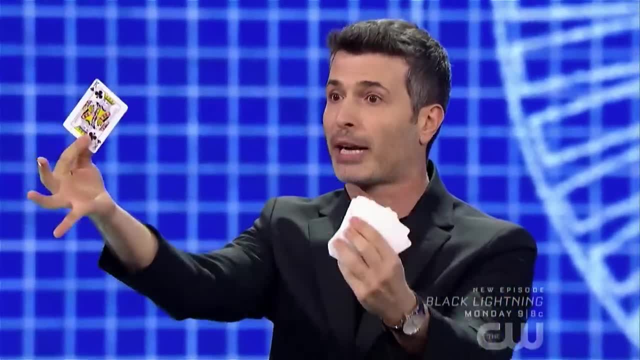 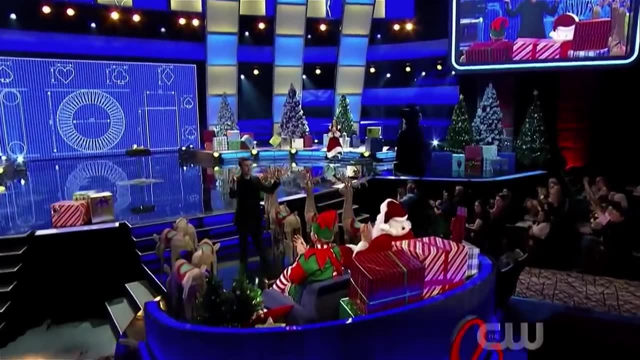 Every one of these cards is a blank card. This is the only option, the only card you could have named, And I know Thank you, I know you love to examine cards, so these are for you. Happy holidays, Enjoy, Thank you. 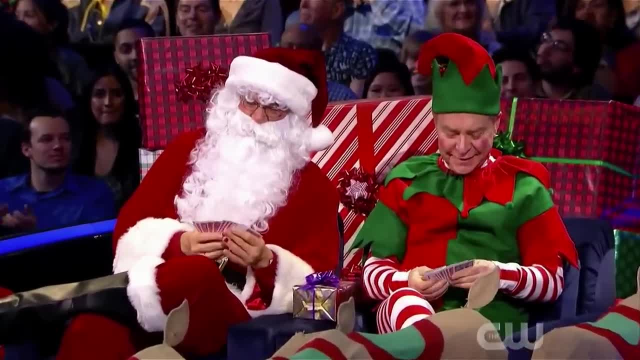 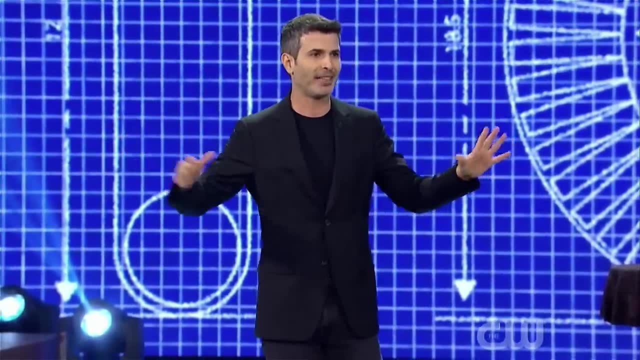 Enjoy yourself. The first time I got Cooled was when I was 13 years old. I went to a magic shop And the man behind the counter showed me the first card trick I've ever seen, And I remember I was in awe. 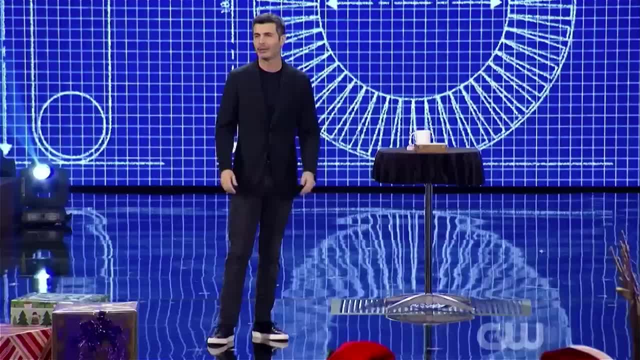 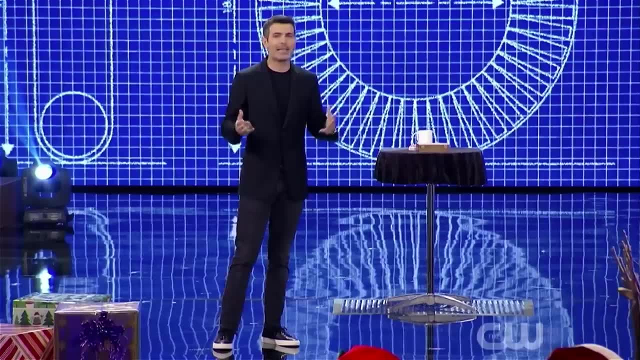 For me, it was a miracle. I said to him: you've got to tell me how it's done. And he said: well, it's impossible, It's against the magician's code, But I can sell it to you for 50 shekels. 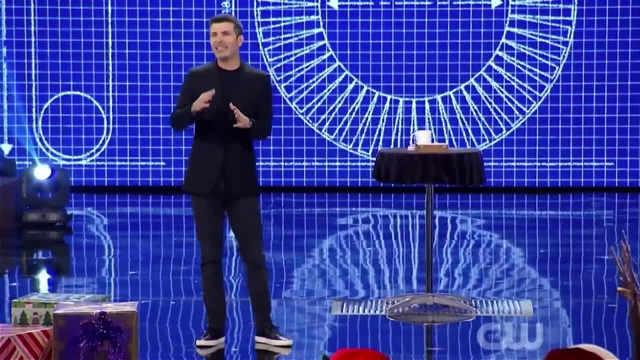 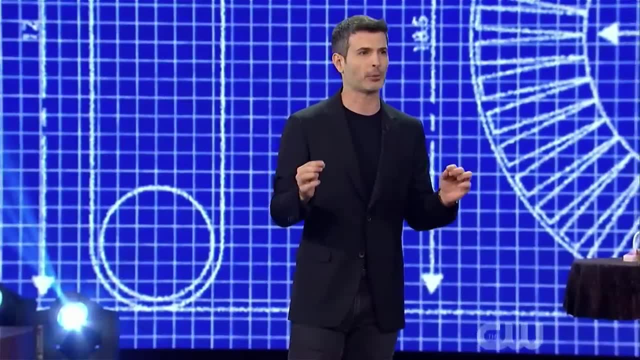 I said, okay, I'm buying it. I bought the trick, learned it And years later I realized that, even though I learned a great trick, I lost something in that store. I lost the mystery. I could never see the trick again. 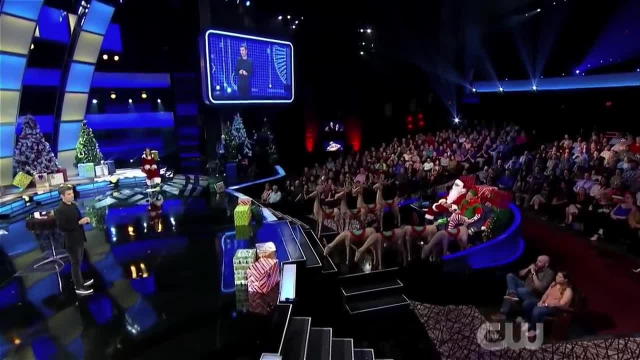 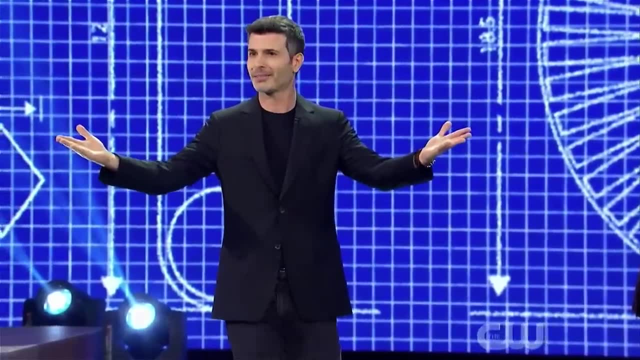 So I'm going to explain this trick to you, But keep in mind that once I show you how it's done, you can't unknow it. Do you still want to know how it's done? It's going to be 50 shekels a person. 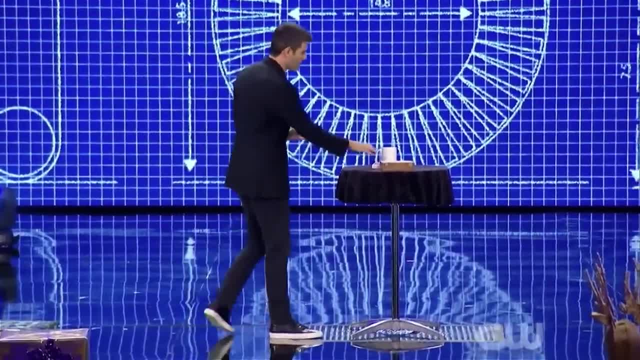 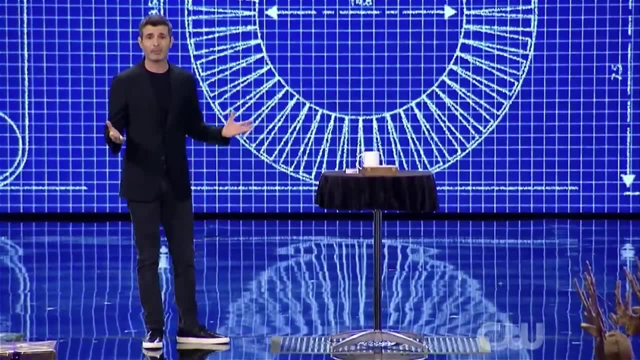 All right, It's the holidays, It's on the house, So, first things first, You have to remember that everything on stage is a part of of the illusion. Nothing is innocent, Nothing is as it seems, Because my goal is to create a moment that has no explanation. 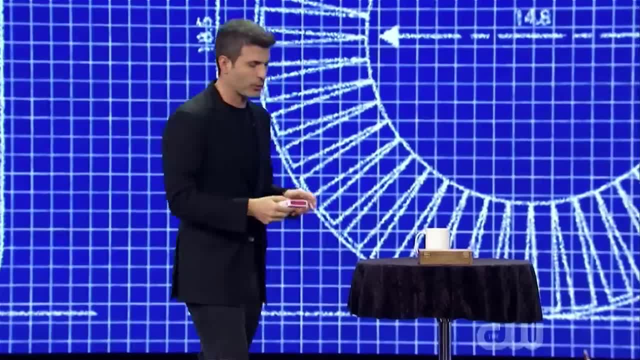 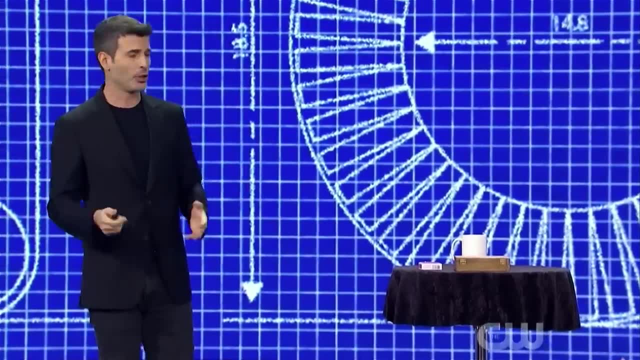 No explanation. So the first question you want to ask yourself is: why did I place the cards inside a wooden box and not just right on the table? I did it because I had to, So let's replace this box with a similar box made of clear plastic. 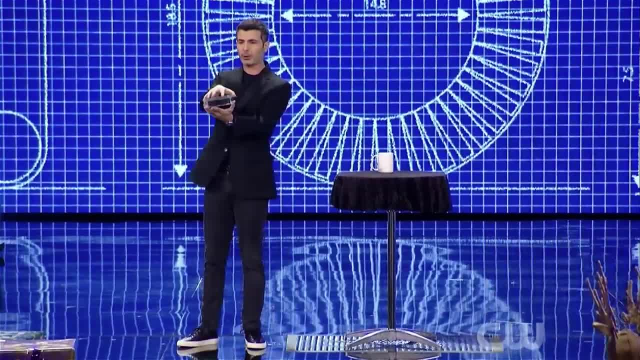 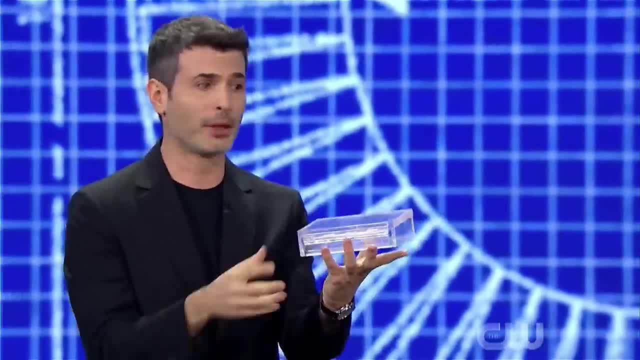 And it's very, very similar, But what's special about it is that when you open the lid, it lifts the bottom with it. Okay, So there's a little bit of a path. Also, there are magnets on the bottom of this box. 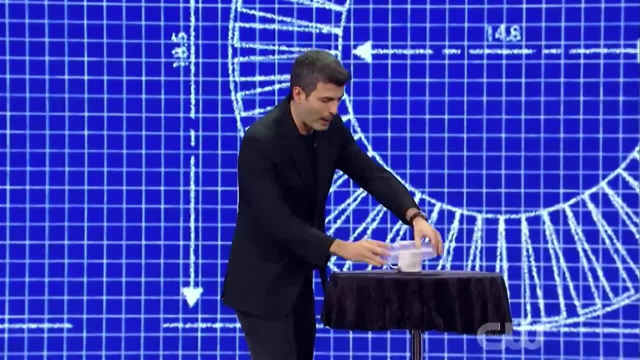 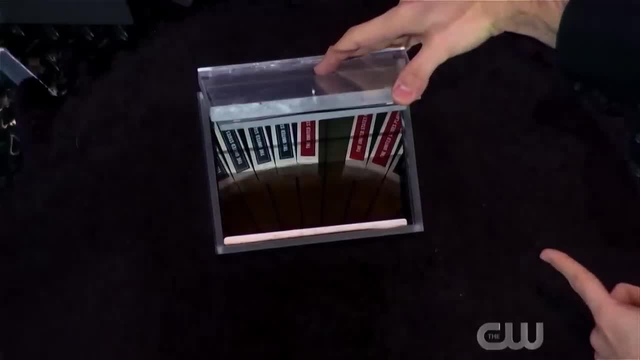 And this table has a trapdoor, So when I place it right above the trapdoor, when I open it, it will open the trapdoor with it And you can see that inside there's decks of cards. Yes, decks of cards inside. 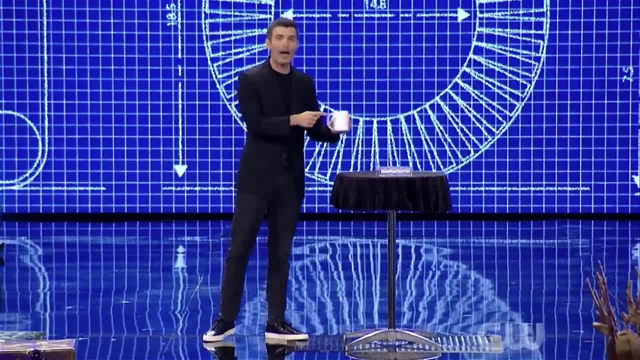 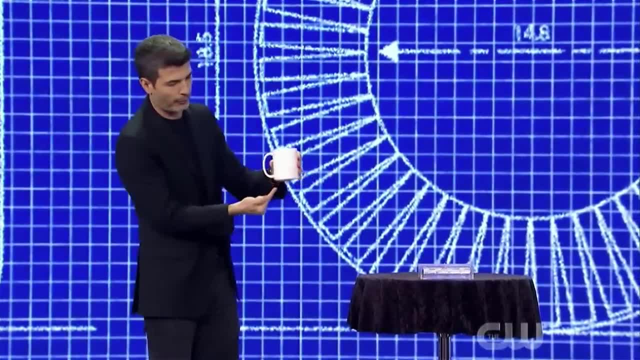 Now, at some point, if you remember, I was drinking. Why did I drink? I did not have to drink, I drank because I had to for the trick to work. You see, this mug has a little bit, Four magnets on the bottom. 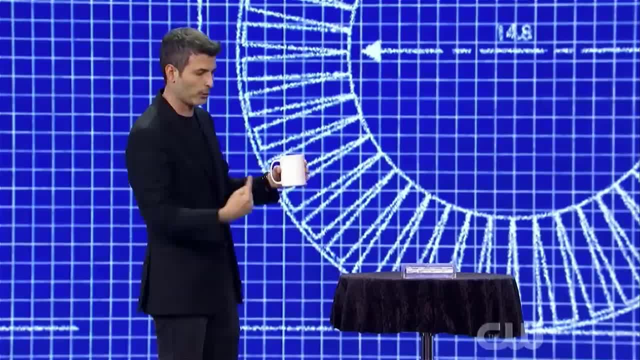 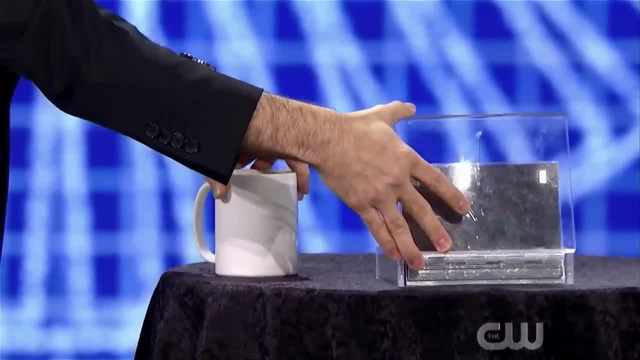 And underneath the surface there's a disc, a circular gear. So if I place it right about here and if I now turn the mug, it will cause all the decks inside to rotate. Okay, You know what? Let me just give you a much better view on this. 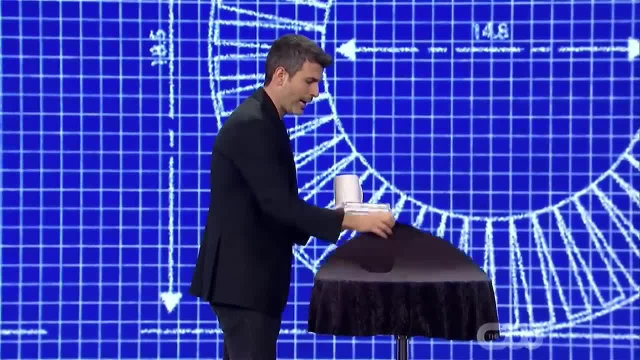 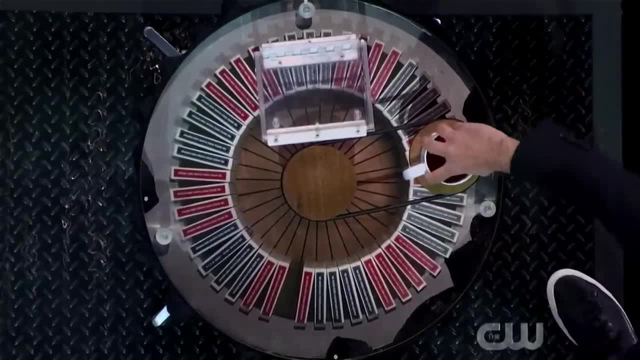 so you can really understand. This is a very strong magnet, So you understand how this really works. As you can see, you have all the decks in there, And when I place it right about here and rotate that, then in every one of the 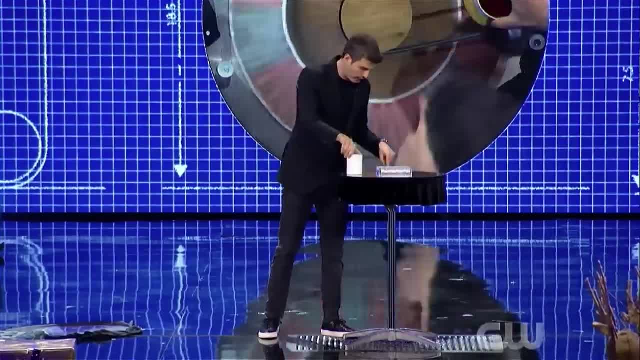 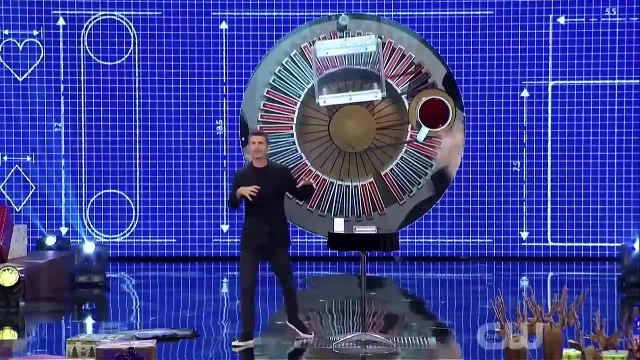 52 decks. there's one card reversed And obviously I took, as you can see, one deck because that was the card you named, So I had to take that one, And every other deck has one card reversed. Do you see how this could help you with the trick? 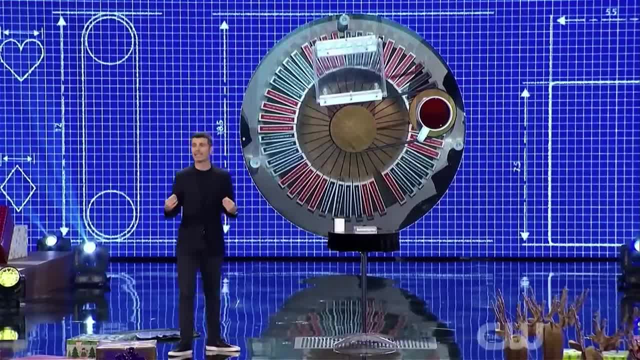 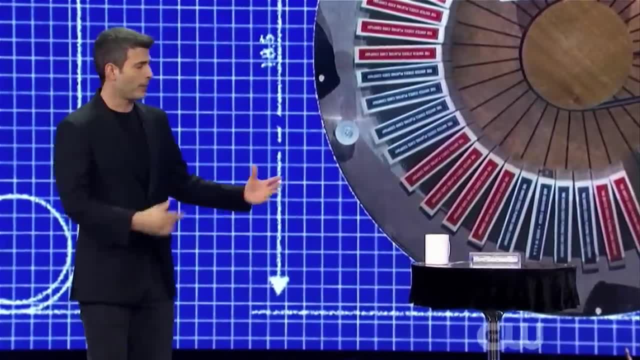 I wanted you to feel for a brief moment what it's like to be on my side of magic For a brief moment, to enjoy the part that I find beautiful. But I did not want to. I don't want you to pay the price I paid. 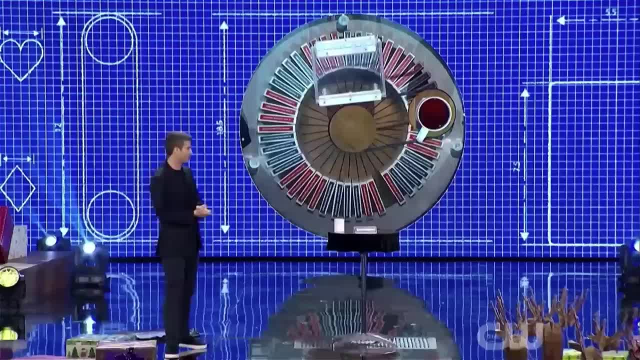 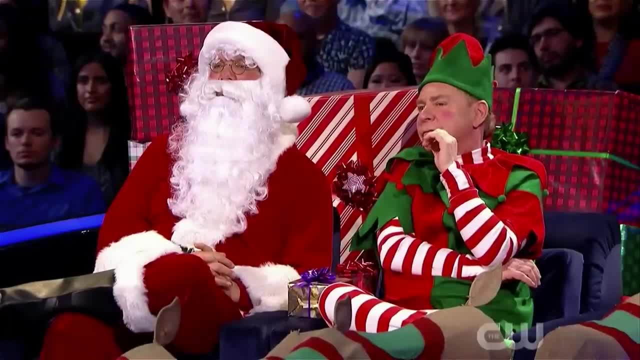 When I lost the mystery, I could not see the trick again. I made a choice. I chose to learn the secrets. But you didn't, And I can't make that choice for you. That's why I told you at the very beginning: 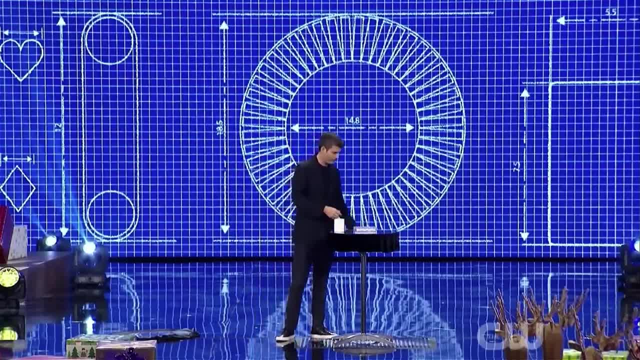 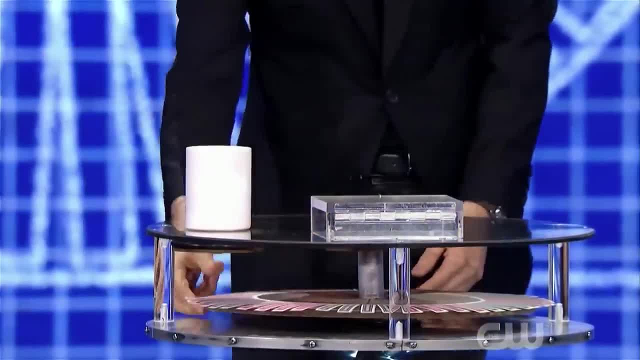 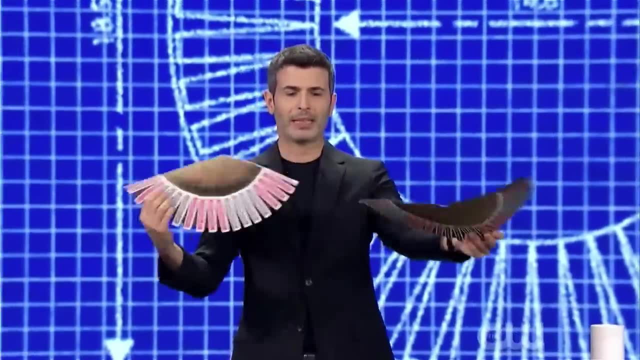 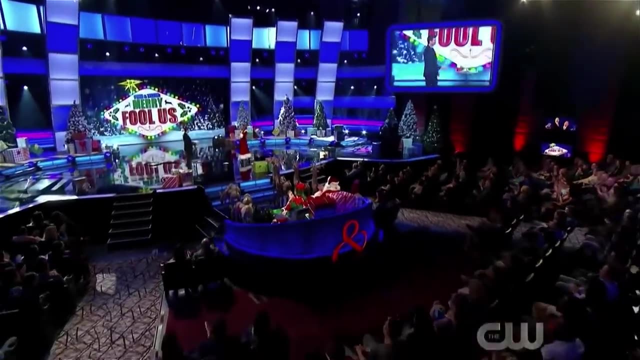 that everything on stage is a part of the illusion. Nothing is innocent, Nothing is as it seems. Thank you. Oh, CLM, I love it. Wow, That was incredible. Thank you. So you do all kinds of tricks. 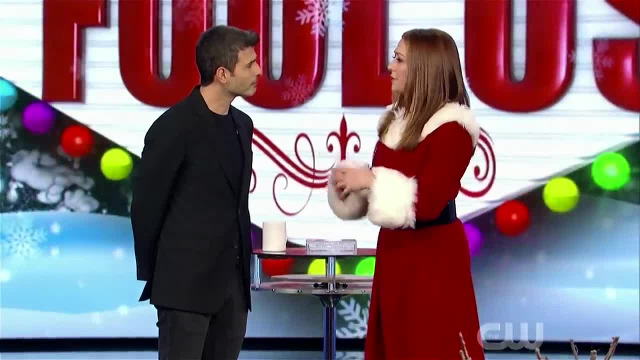 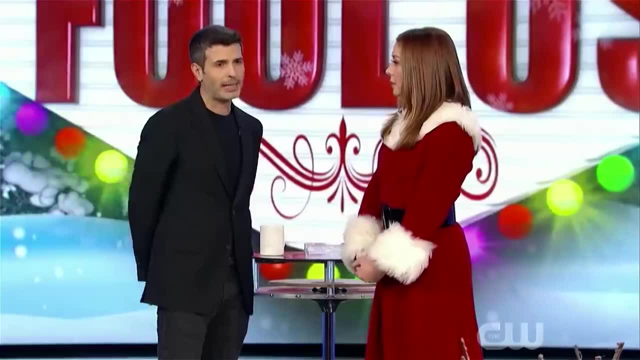 Yes, You come up with tricks. You do tricks. You make up tricks for other magicians- I do. How do you decide which tricks you're going to keep and which you're going to give to other people? I keep the goals for myself. 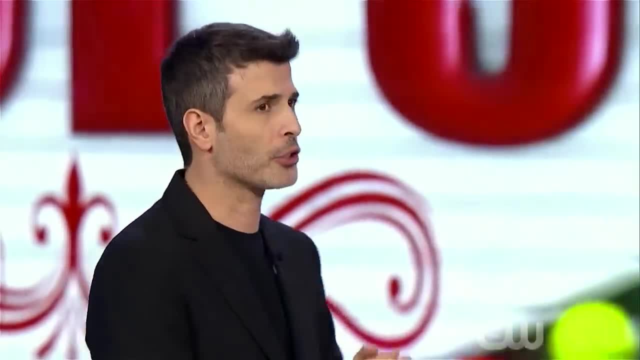 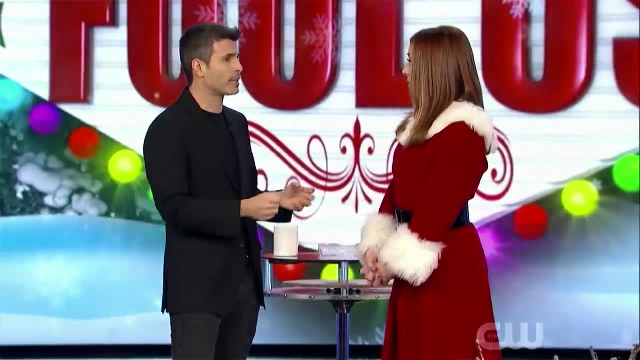 No, actually it's a personality thing. I know there's a trick that they say, wow, that's a great trick. It will never work for my personality, for my type of show, Or sometimes it's just by design. Somebody wants a specific trick. 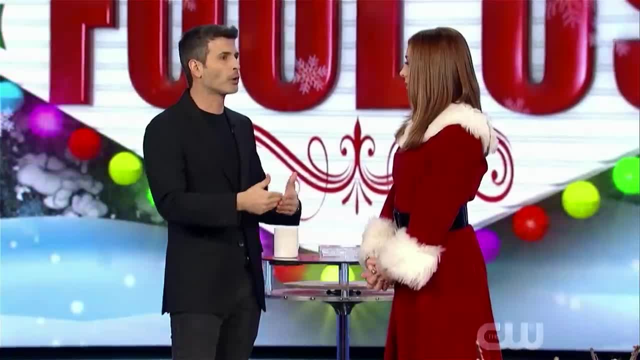 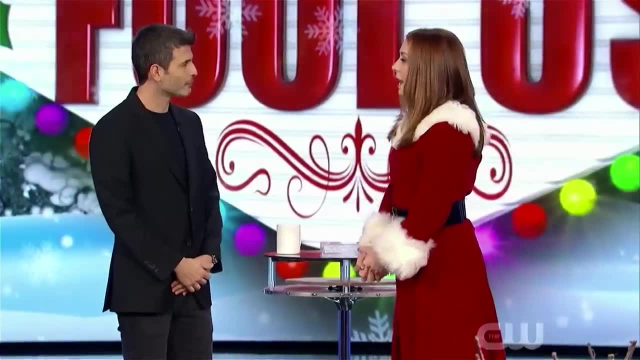 and I say, okay, how do we achieve that? And then I work with that person to create that moment. So it's a collaboration more than anything, Of course. That's amazing, Thank you. Have Penn and Teller been an influence on you? 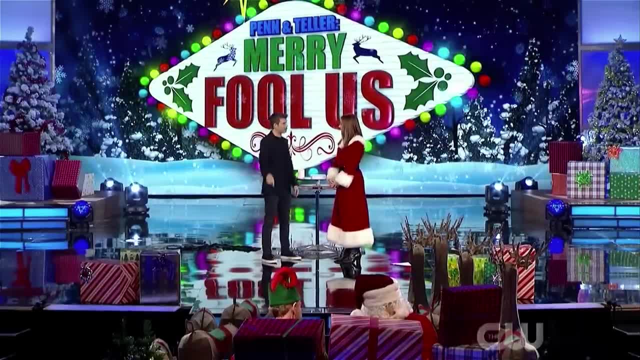 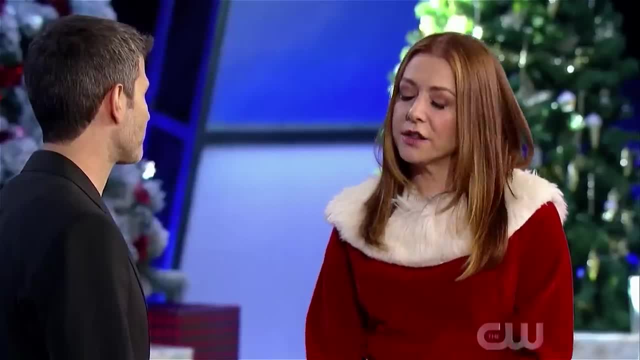 I think there's some fingerprints on this thing that are very much influenced by Penn And Teller, but also by one of my favorite magicians, Tommy Wonder, and many others, of course, And are there like magic tricks, you'll see. 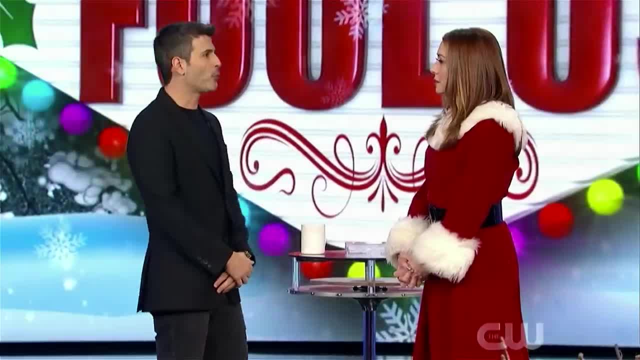 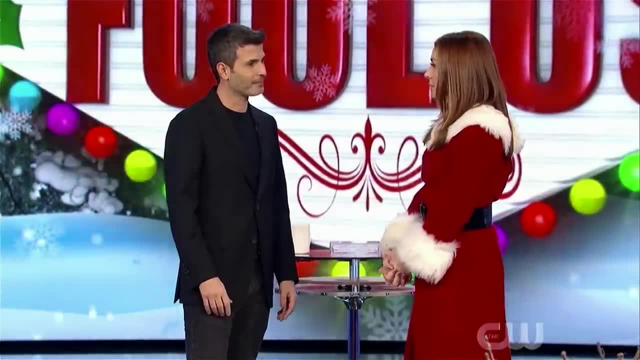 and you can't figure it out from other magicians. Unfortunately it's rare. I want to, I like to be fooled. Is there at least one that takes you a long time, Because I've seen them. when somebody will fool them. 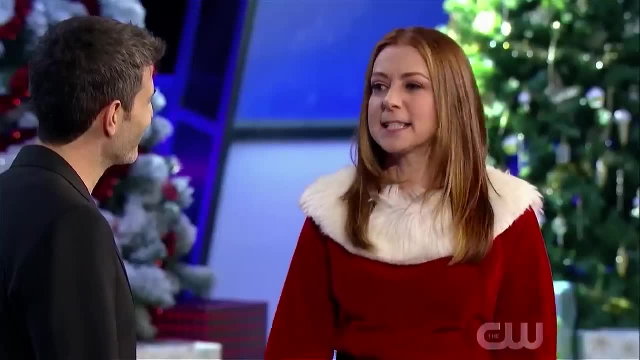 they get so angry and they walk backstage and they're like you have to tell us how it's done, But it's a good anger, It's a good one. No, exactly, It's the only kind of anger you want, That you want to have in your life. 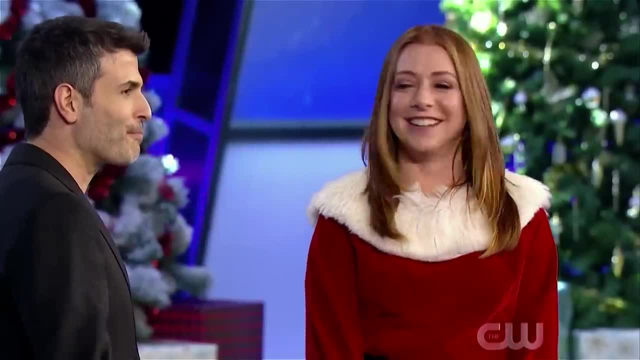 But they can't stand it. It's so exciting, It's really fun. They're like. you have to tell us They're different. It's so cool. Well, I was astonished. Let's see what Penn and Teller thought.